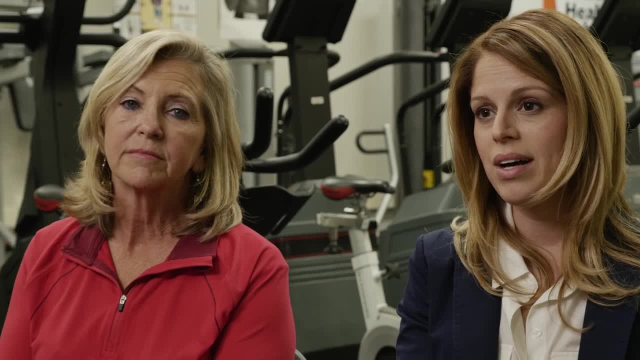 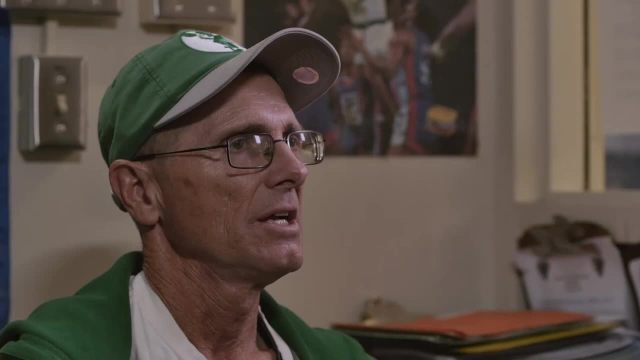 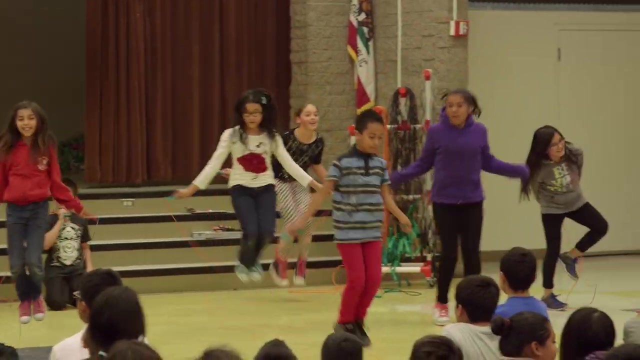 and Loma Vista is one of them. They are one of the healthiest schools in the US and they're just a really special place for kids to be. First of all, we changed the whole idea of PE. We're teaching kids about activity, not sports. that will lead to healthier living. 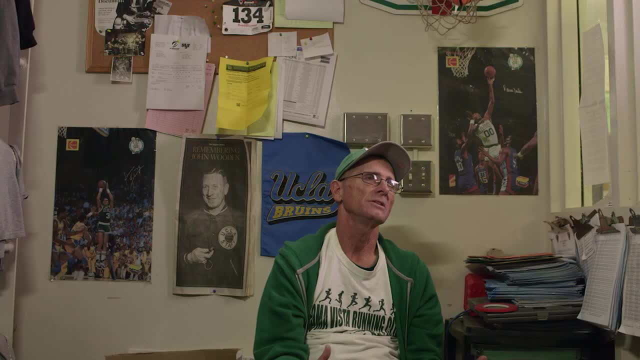 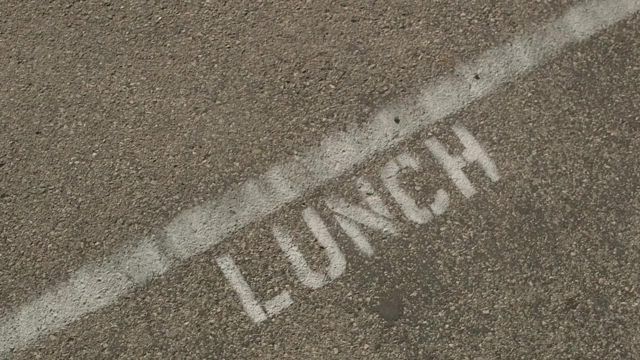 You need to eat the right way, You need to get the sweep you need. You need all those facets. You can exercise all you want, but sooner or later it's going to come down to eating. It's all about choices, and we make good choices, we make bad choices. 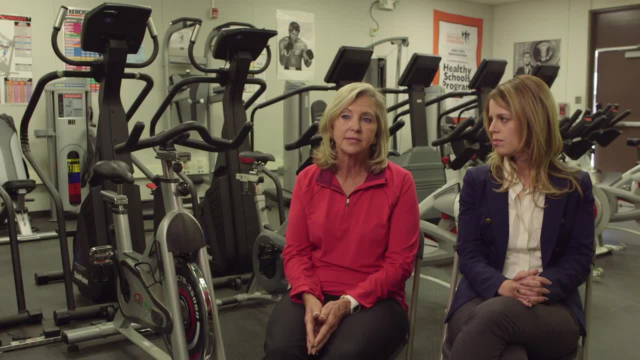 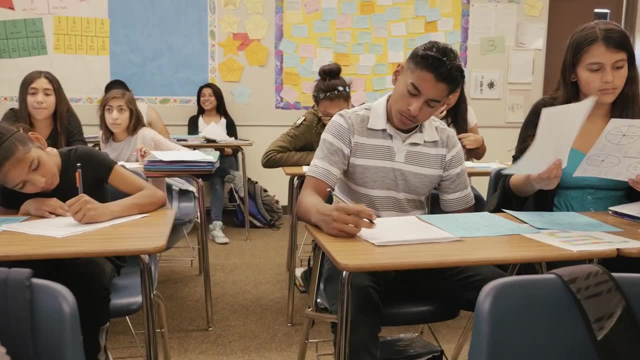 But the bottom line is they have to be given the education to make those choices, and that's what we're here for. So we have nutrition education in our classes. We try to help the kids learn what is healthy choices for food When they go home. we can't control what their parents are going to feed them. 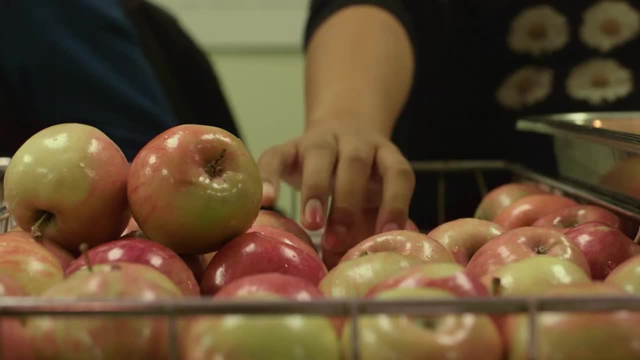 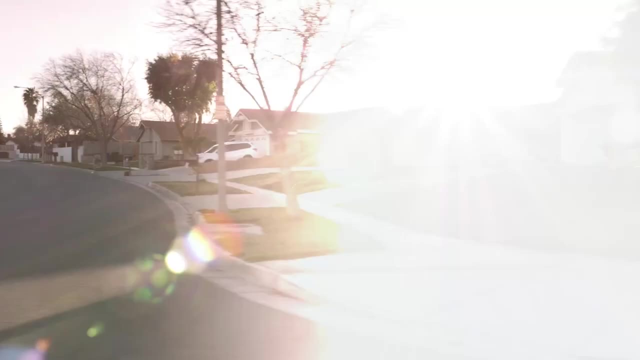 but hopefully the kids will step up and say: Hey Mom, how about this? Why don't we try this? I would say the biggest task is the parents. We come from an area where a lot of our parents either work two jobs or they're gone when the kids come home. 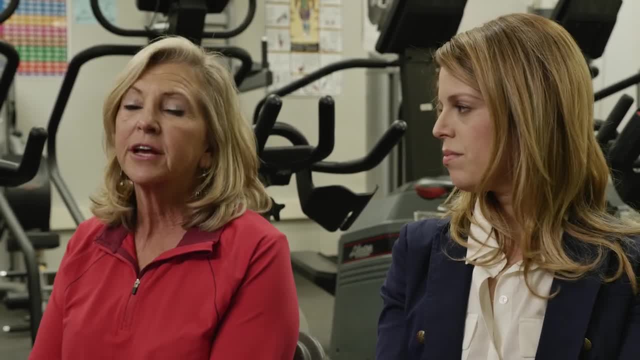 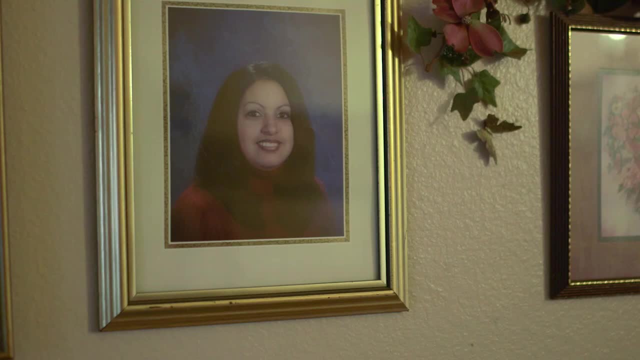 So the kids will grab something quick and easy. The parents fix for them something that's quick and easy, or stop and buy something. I don't know anybody in this family that has ever been naturally skinny, but like my mom. when I see her eat junk food, that's all I think about. 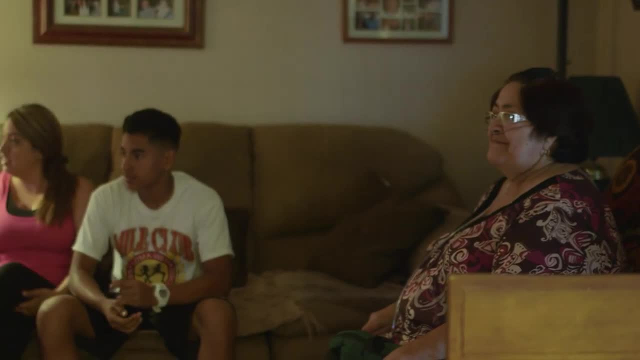 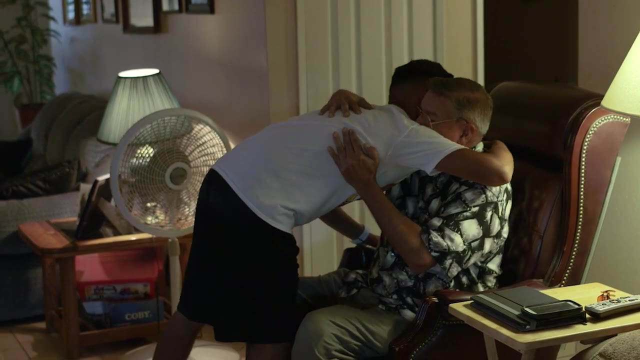 That if she keeps doing this she's going to turn into a diabetic. Oxygen means she can't breathe, right? You ask the kids how many of you have a family member who's had a heart attack And you're going to see 75% of our kids raise their hand. 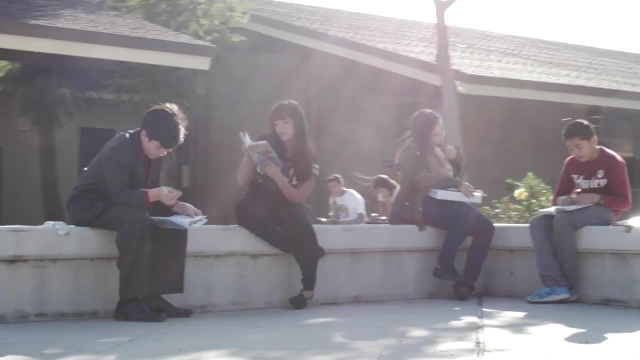 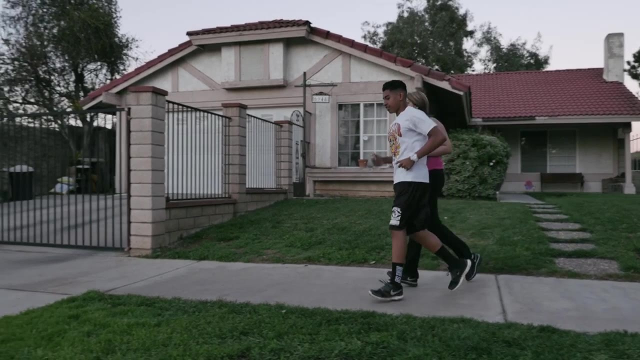 That's going to be the future of our children if they don't make some wise choices. We're trying to get that message across to them so that future generations of their kids will maybe turn it around. I just want her to stay healthy. She's my mom. She gave birth to me. 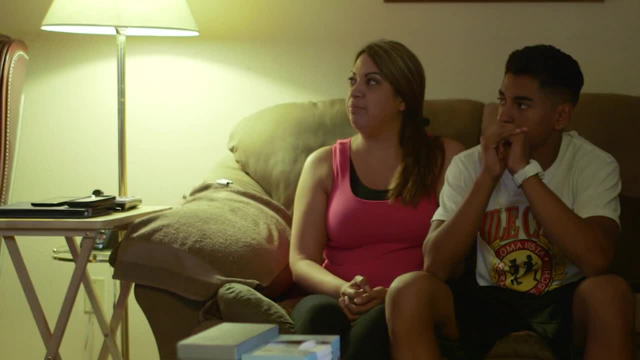 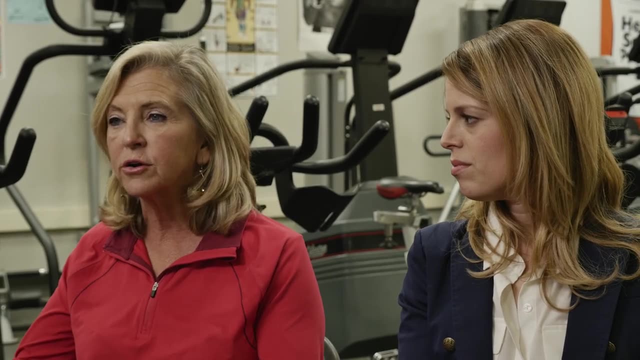 When I think about community, I think about the parents, the teachers, the students and all of our community members, Kaiser Permanente, all of our partners that join with us. We have partner meetings a few times a year where they all come together and talk about.